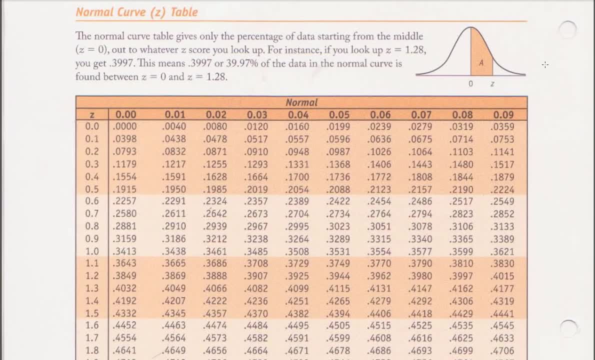 Hi guys, in this video I'm going to introduce the normal curve table, or sometimes just called the Z table, and basically this is one of many versions of the table that we're looking at right now. This particular table can be identified by looking at the picture on the top right over here. This picture: 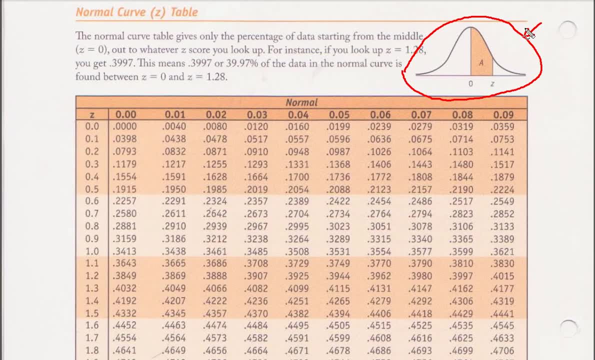 tells us which of the many different versions of normal curve tables or Z tables we're looking at. So I'm going to be using this particular table for many of the exercises that I do on normal distributions from here on. So if you want to follow with me, try to grab this version of a normal table Now every. 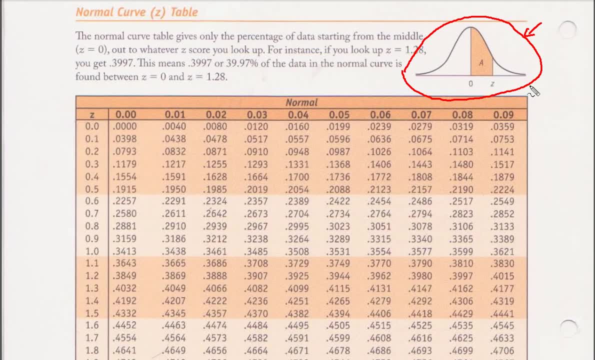 textbook- statistics textbook- you're going to want to grab this version of a normal table. This textbook has a few tables and also you may be able to find them online as well. So if you want to do it the way I'm with the table that I'm using it, this is the 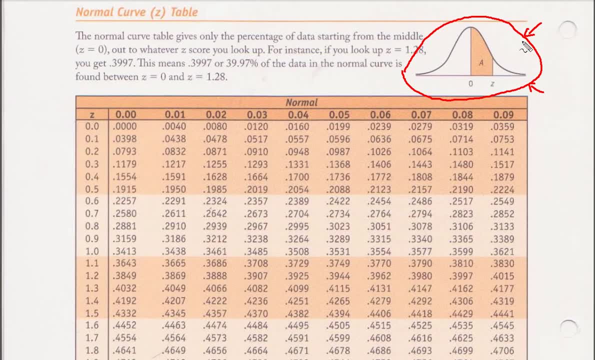 table that I'm using. Sometimes it doesn't show you a picture and it writes something. This table writes something and draws the picture, So let's see what it says. It says that this normal curve table gives only the percentage of data starting from the middle Right. this is the percentage of data starting from the middle. 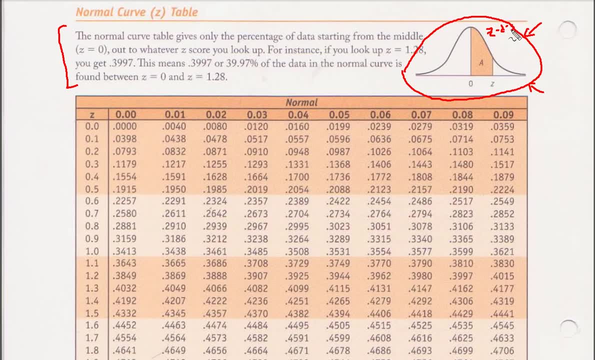 This is the Z distribution. So remember, mu is equal to 0 and Sigma is equal to 1.. This is the standard normal distribution, Right, standard normal. So there's many normal distributions, each distinguished by mu and Sigma: Right, the mean and the standard deviation. The mu when mu is 0 and Sigma is 1.. The normal: 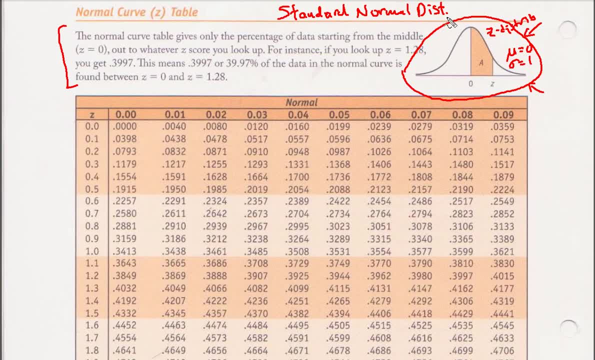 distribution is called the standard, normal or Z distribution, And that's what all the tables are showing you. Okay, notice these Z values here. Okay, so let me continue Then, don't? this table gives the percentage of data starting from the middle. Z equals 0 out to whatever Z score you look up. 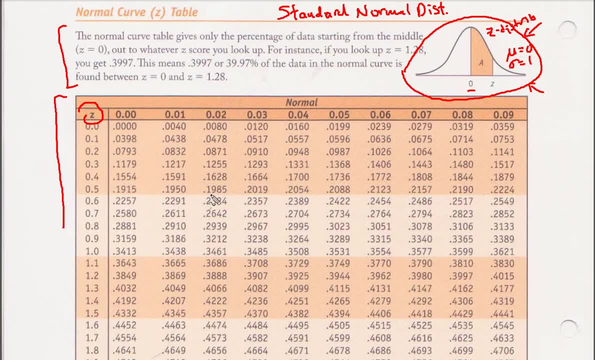 So, for instance, if you look up 1.28- and we'll go down here- here's 1.2.. By the way, the Z's are in the first column and first row. So when you're looking up a Z score, you look at the first column and first row. Inside here are the 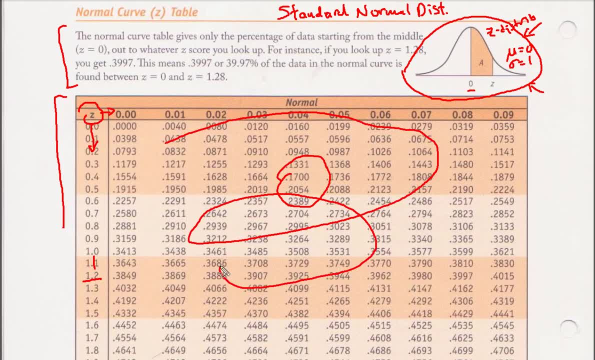 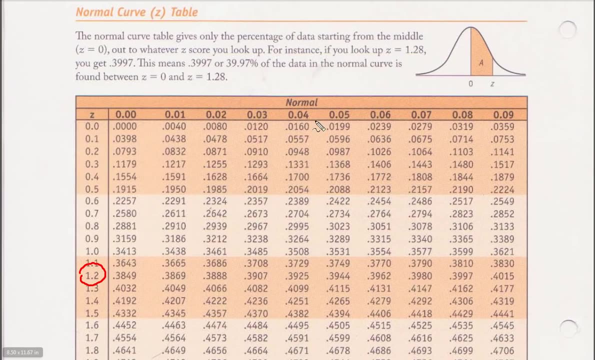 percentages. Basically, all these guys in here are percentages. Okay, so let's say we're going to look at the bottom here, Right, this is going to be the first column, and then we're going to look up the bottom up. for instance, z equals 1.28. so we look up 1.2. it's a Z right, so 1.2. and then we 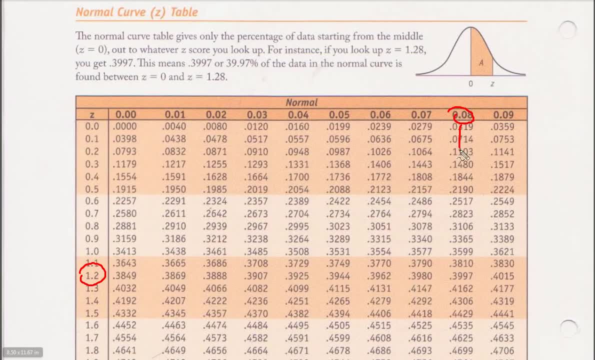 need the 0.08 part, and what we do is we kind of square in and we get the percentage of data right here. okay, now, what is this percentage? let's go back. this table tells us the percentage from the middle to a Z value that you look up. 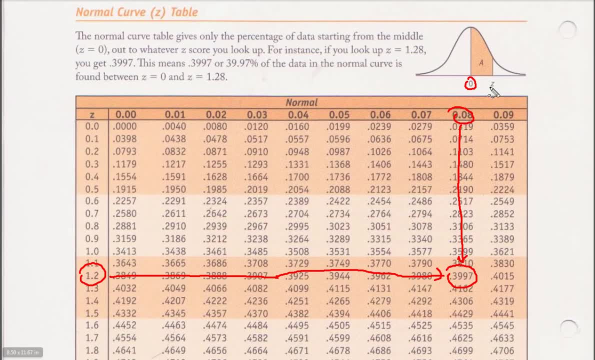 a Z score. okay, so since we looked up 1.28, that's what we replace that Z over here in the picture with 1.28 and what we got is that 39 right here. 39 point nine, seven percent of that point seven percent of. 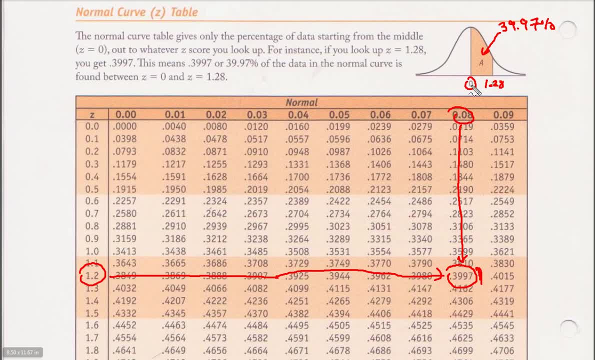 of the data is between z equals 0 and z equals 1.28.. That's how this table works. So if you're using another table, just be familiar with how your table works And always remember to, at least in the beginning. 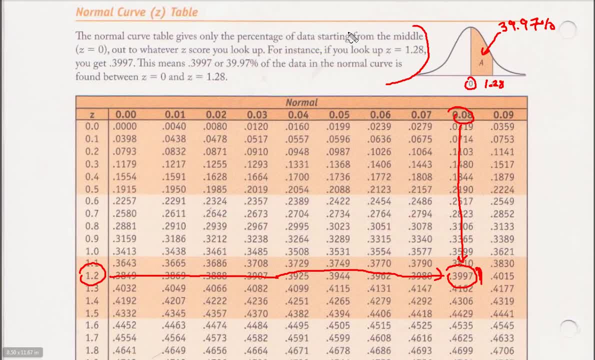 to either read which table you're looking at or look at the picture to remind you of what these numbers in here are telling you, Because if you just blindly go and look up z scores, you're going to get percentages that don't necessarily correspond to the areas that you're looking for. 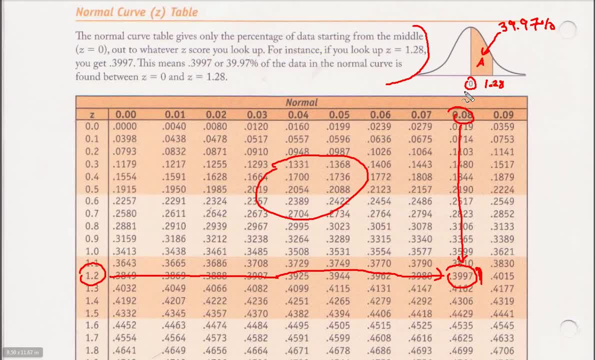 By the way, this A stands for area because, as we'll see in further examples, the area under the curve, which is represented by this shaded orange region under the curve between the values that you're interested in, that's an area right. 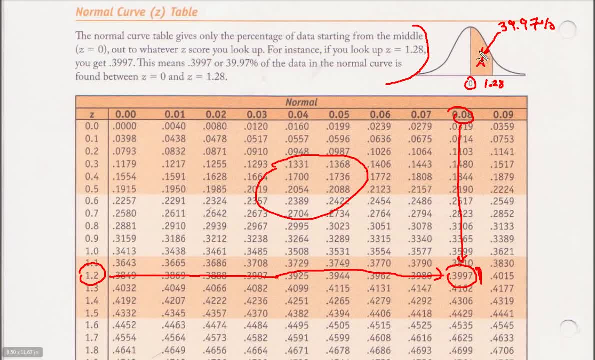 That area is equal to The percentage of data between these two values here. So area percentage, probability proportion- these concepts kind of merge together when we talk about normal distributions. So questions can come in many different ways And we're going to do a bunch of questions. 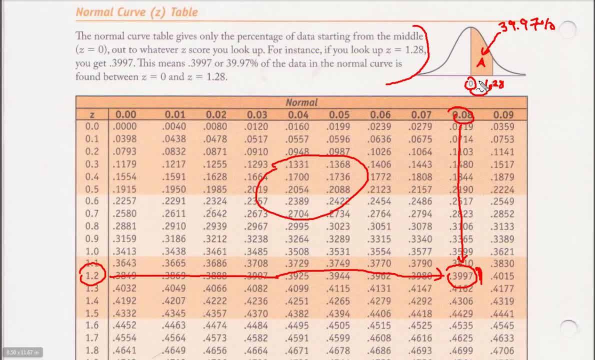 I just wanted to start this video for you to know how to read a table, and we're going to definitely have learned more about this table as we answer more complicated questions. But this is the basics, the fundamentals of the table that I'm using. OK. 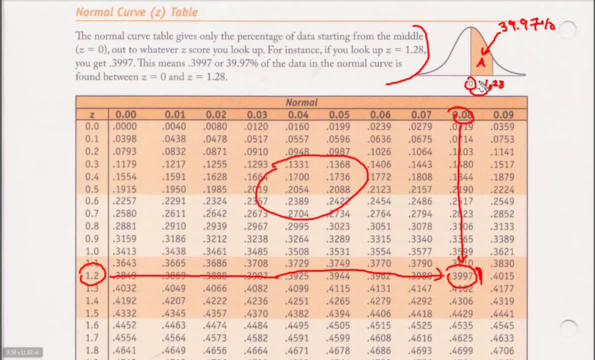 All right, so be sure to watch the following videos where I'm going to actually do examples with normal distributions. OK, Until next time, have a great day. 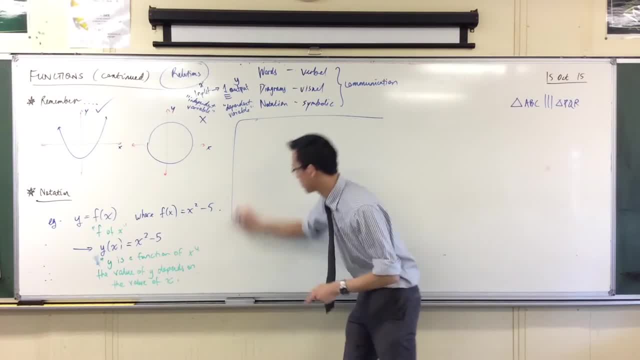 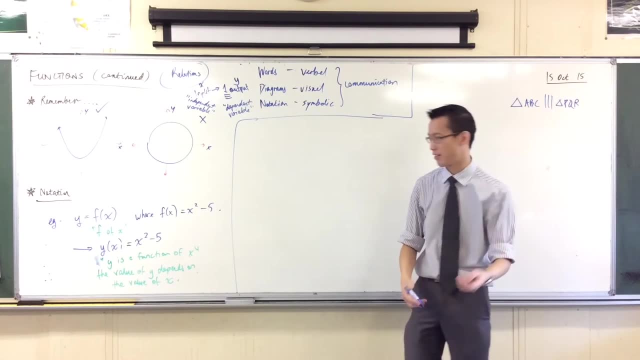 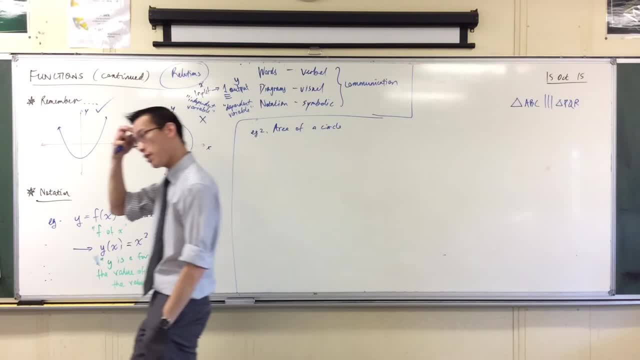 you guys know there's a formula for the area of a circle, right? But the formula is just a function, right? It's just a connection between area and area and what. What's the other variable it's connected to? It's just radius, right.